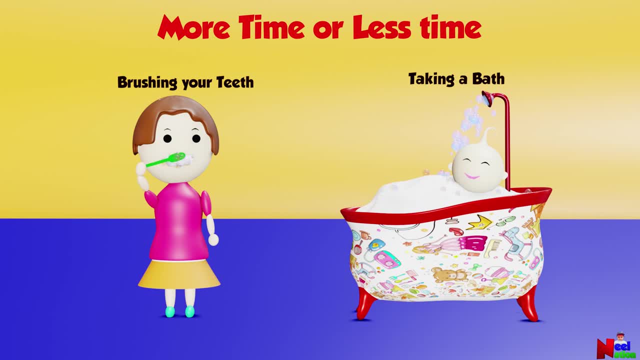 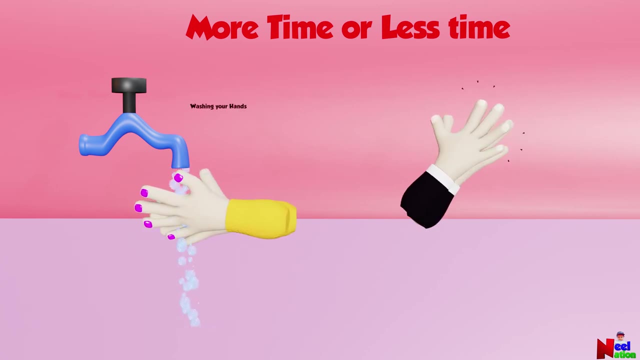 Brushing your teeth or bathing? Brushing your teeth takes less time. Bathing takes more time. What takes more time and what takes less time? Washing your hands or clapping? Washing your hands takes more time. Clapping takes less time. Yes, Washing your hands takes more time than. 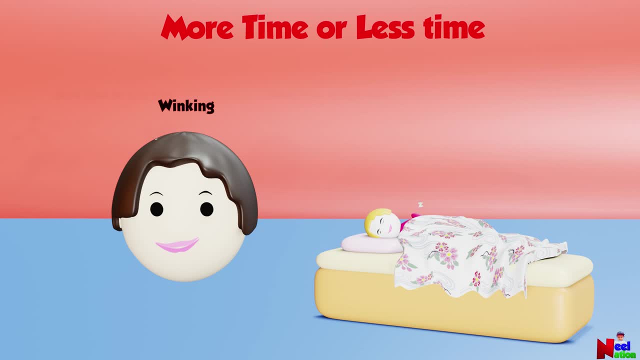 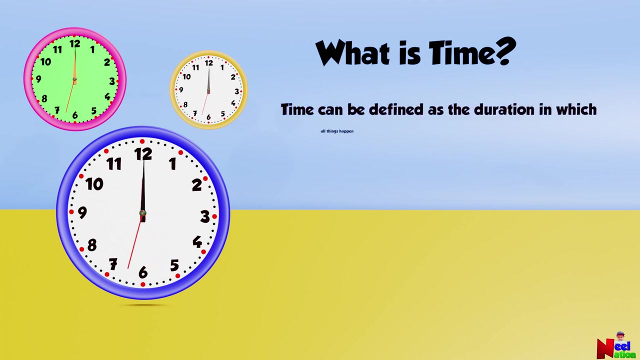 clapping. What takes more time, winking or sleeping? Sleeping takes more time, Winking takes less time. Yes, sleeping takes more time and winking takes less time. So what is time? Time can be defined as the duration in which all things happen, or a precise instant at 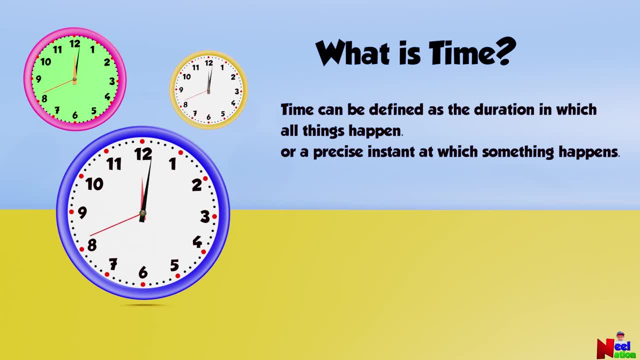 which something happens. The basic unit of time is second. We measure time in seconds, minutes, hours, days, months, years and so on. We measure time using clocks and calendars: Seconds, minutes, hours and days. So let's learn about second. 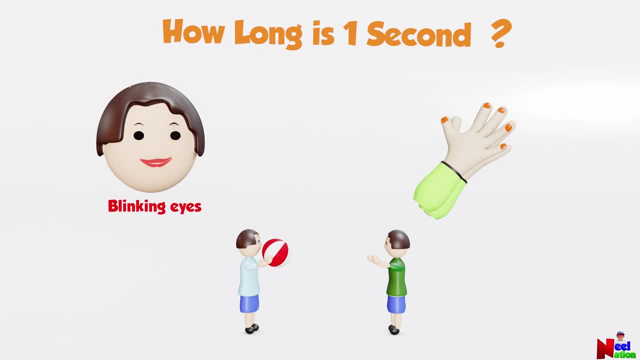 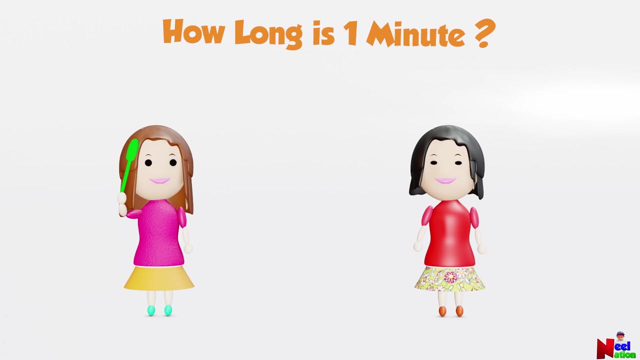 How long is a second? Blinking your eyes: once takes a second. Clapping your hand: once can take a second. Throwing a ball: also takes a second. Now, how long is a minute? Sixty seconds make one minute. Sixty seconds make one minute. 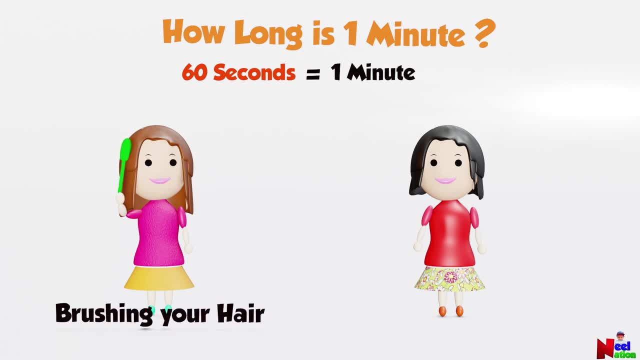 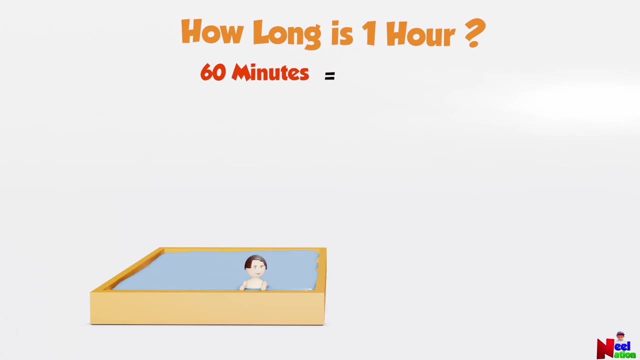 Things like brushing your hair or singing your nursery rhyme could take a minute. Okay, How long is an hour? Sixty minutes make one hour. Sixty minutes make one hour. Your swimming lessons could take an hour, or walking your dog could take an hour. 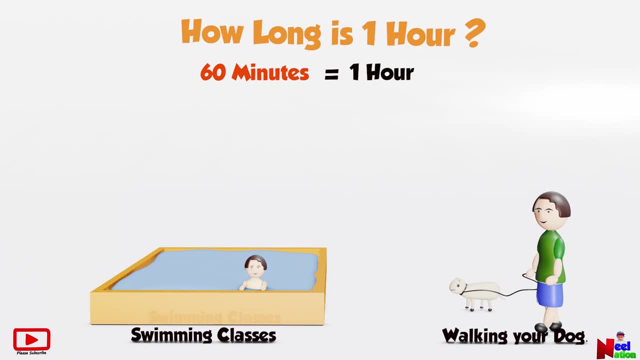 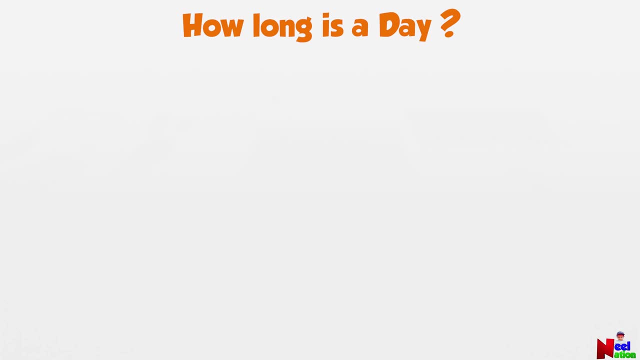 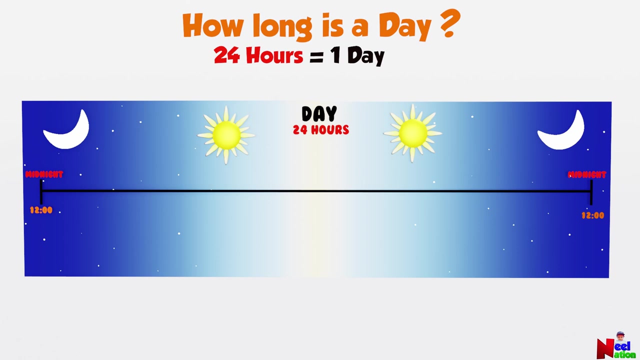 Okay, Next. Now let's learn about a day. How long is a day? 24 hours makes one day. In other words, a day is 24 hours long. A day is 24-hour period, starting from 1 midnight to the next. 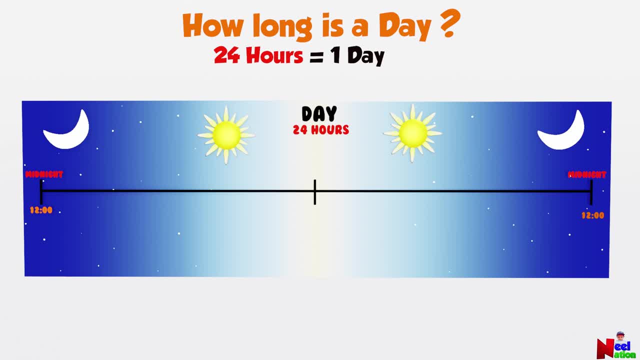 Let's divide a day into two equal halves of 12 hours each. The midpoint is called noon or midday. The first midpoint is called midday. 12 hours is called before noon. We use am to tell time starting from midnight to noon. 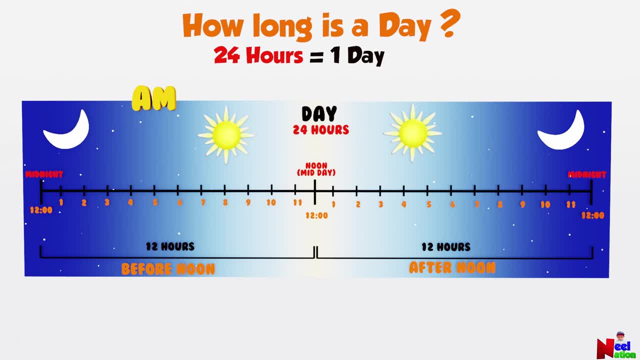 The second half of the day is called afternoon. We use pm to tell time starting from noon to midnight. You might have heard someone say: get ready. Your school starts at 8 o'clock. You wake up at 8 in the morning. that is 8 am. 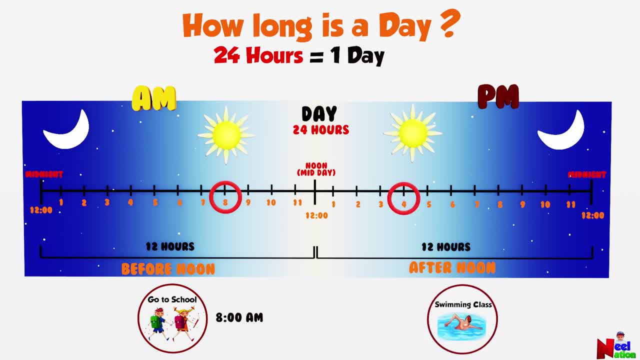 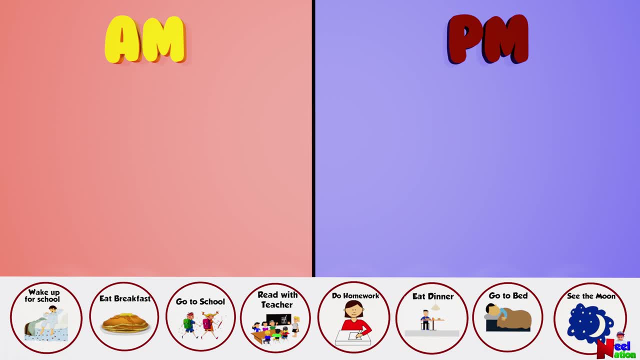 And your swimming classes are at 4 in the afternoon, that is, 4 pm. You do lots of activities in a day. Let's sort them by am and pm. When do you wake up for school In the am? 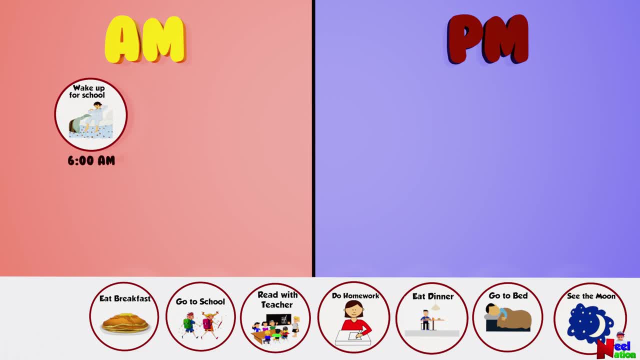 At 6 am. When do you have your breakfast In the am? At 7 am. When do you go to school In the am? At 8 am. When do you read with your teacher In the am? 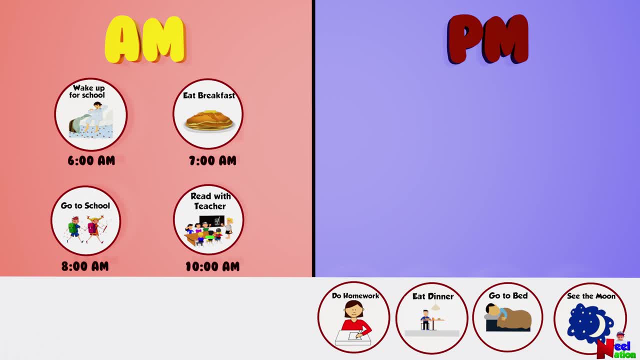 At 10 am. When do you do your homework? In the pm 6 pm. When do you have your dinner? In the pm. When do you have your breakfast? In the pm 6 am. 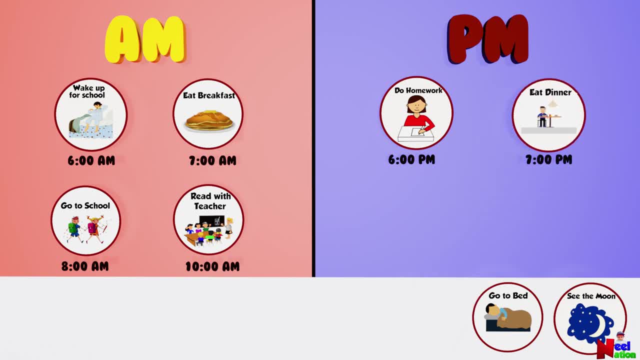 When do you close the door In the am? In the pm 7 pm? When do you go to bed? In the pm 8 pm? When do you see the moon In the pm?